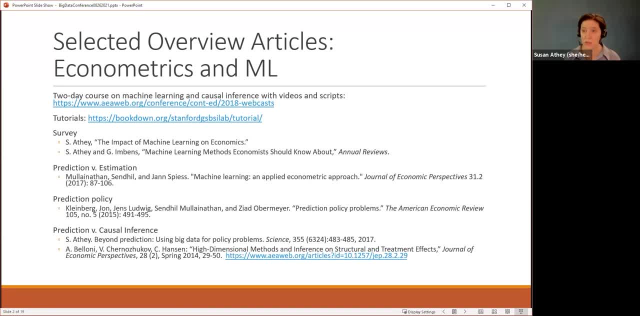 that my slide isn't updated. I have a series on YouTube from my course this year, And then I have tutorials that you can download and run. So it's like a book, but you can, when you download them, you can also run the scripts and modify them and change them, And those 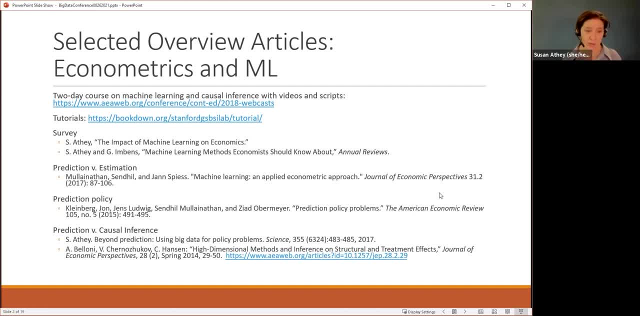 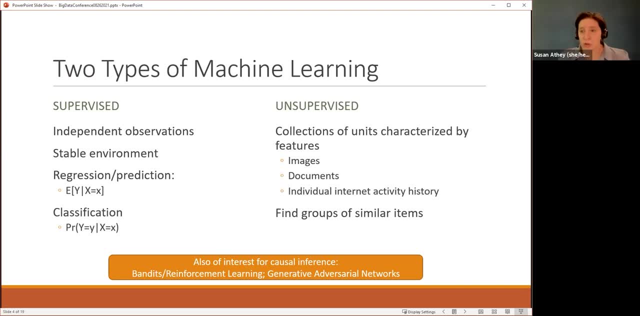 are really focused more on the causal inference side of things, And I have some other references here as well, if you're interested. So first of all, like big picture, you know there are two kinds of machine learning. Really actually there's more, but I think the ones you're most likely to first encounter fall. 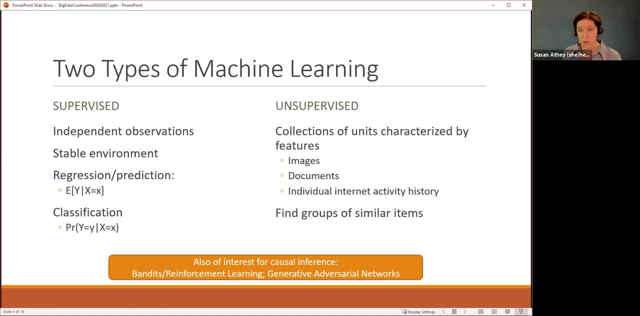 into these two buckets And I'm going to focus mostly today on supervised machine learning. And so supervised machine learning is set up to solve the problem where you have independent observations and a stable environment And then you're trying to do usually one of two. 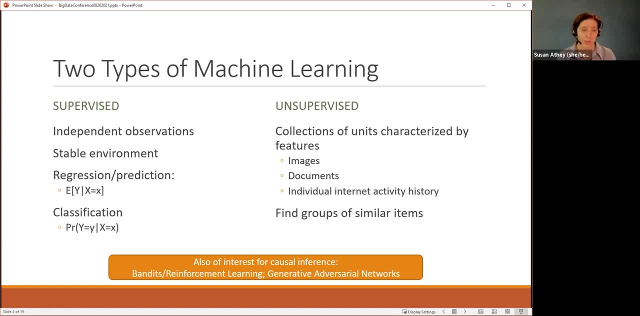 tasks. One is to do some kind of regression or prediction problem, And the other is to do classification And they, you know, the main difference being that the outcome is either continuous or binary, or, you know, can be, or discrete And so supervised. 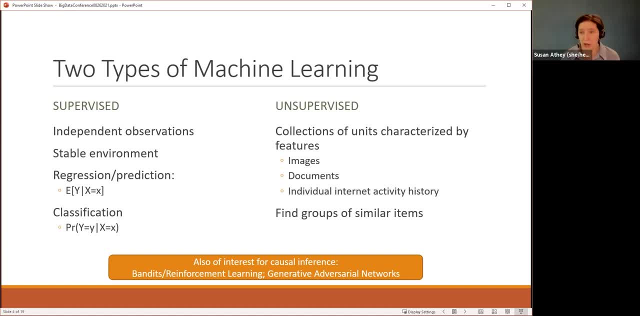 is going to look a lot closer to what you would learn about in a normal econometrics class, And so that's where I think I'll have more insights in terms of trying to draw connections between how we think about what looks like the same problem in the different fields. 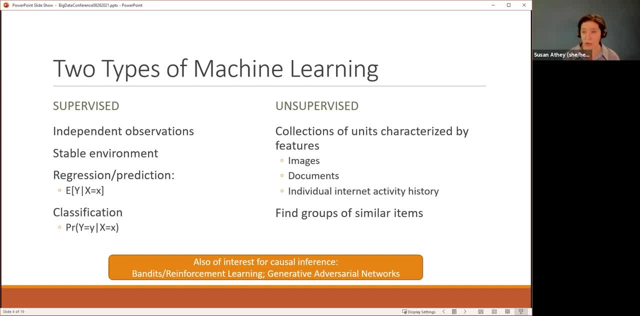 Another part of machine learning that can be very relevant in some parts of macro and finance is unsupervised machine learning. In unsupervised machine learning, you are trying to take objects and put them into groups without necessarily specifying, like prior information about you know- what the what's important or what you want those groups to look like. 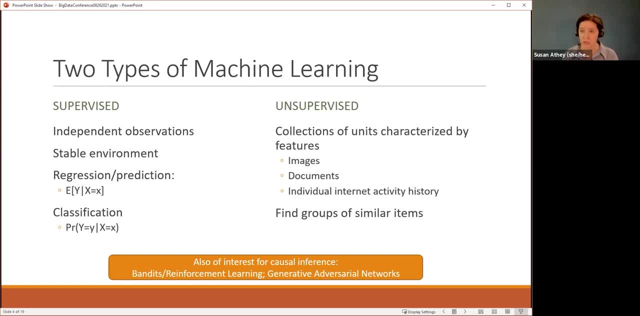 So for unsupervised learning, it might be that, you know, I just take a bunch of text and a bunch of different documents and I say, you know, tell the algorithm, put them into groups. Then, after you put them into groups, you can go back and read the documents and say, oh, you know. 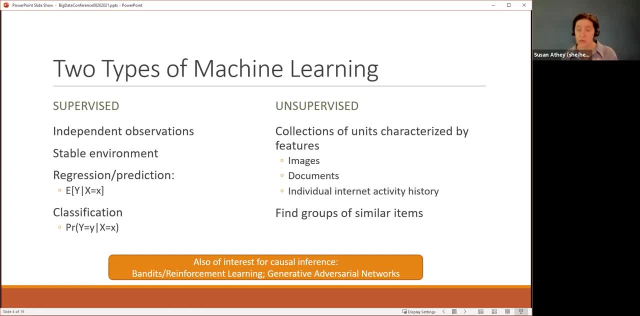 these are new stories about earnings announcements or these are new stories about you know macro events And you can. you can label them afterwards as a human, But you didn't tell the algorithm to go and look for a specific kind of story. You just told it to find things that were similar. 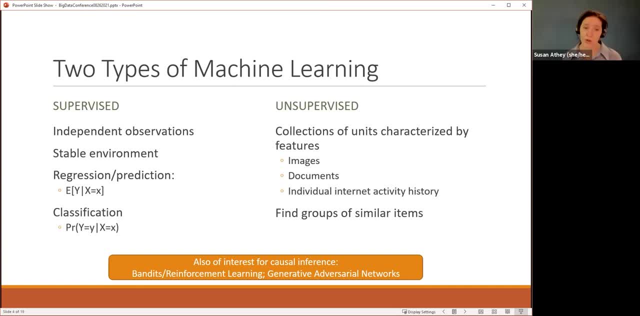 And then there are there are kind of hybrid models where you are trying to kind of reduce the dimensionality or kind of find common themes, but find the themes that are important for prediction or classification, that would that would really be fall into supervised. So I think 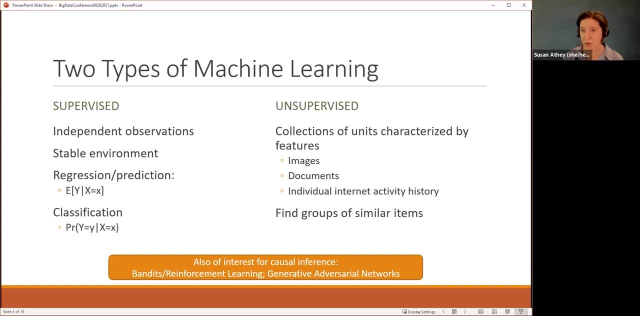 a lot of times it actually can be better to do something supervised if you can. So if your goal in the end is to, you know, figure out how news articles relate to stock prices, then you might find something about you know, find some kind of 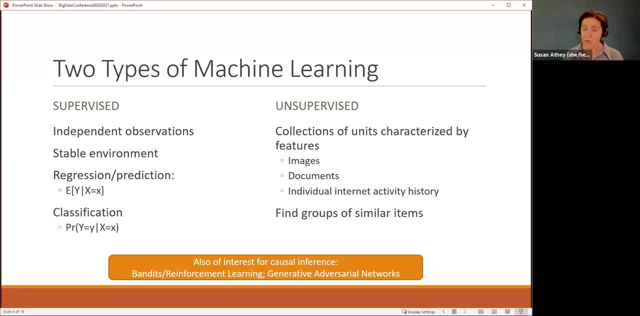 outcome that relates to stock prices, And and then, when you try to to kind of reduce the dimensionality of the text you're reading, you want to find those aspects that are important for solving a problem like predicting stock prices or whatever it is you're trying to predict. 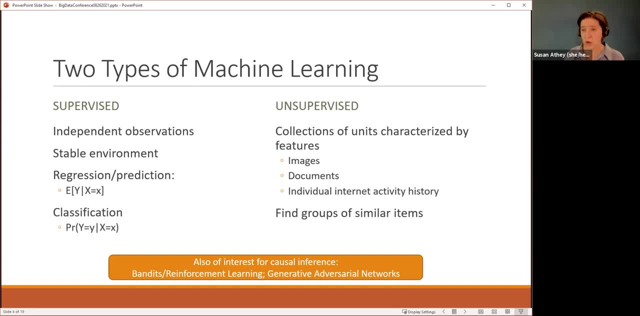 And the challenge with doing unsupervised learning just on its own is that you know we don't have a great way to know when you've done a good job and you know it could be that things are very similar. You can find a group of articles that are similar to each other, but maybe in some dimension. 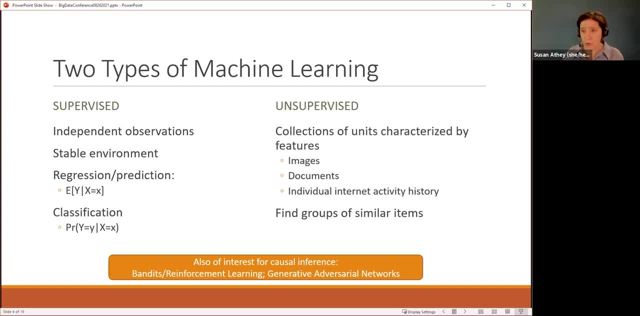 that's not really important for the problem you're solving. People sometimes go off and do unsupervised learning without touching any prediction problem, because they want it to be sort of clean and separate. So they want to say: you know, I don't want to worry that somehow. 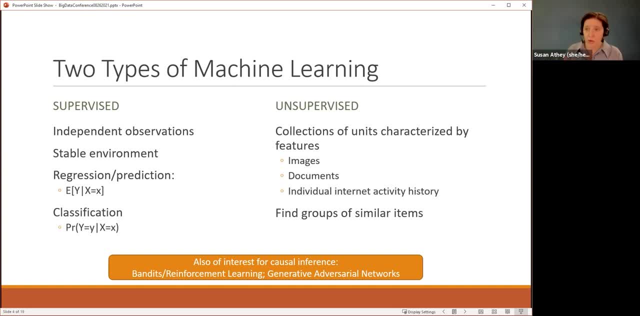 the way I put articles into groups is contaminated by you know some kind of macro variable or something. So that's one. one reason You might do the unsupervised learning, One reason I don't go a lot farther with unsupervised. 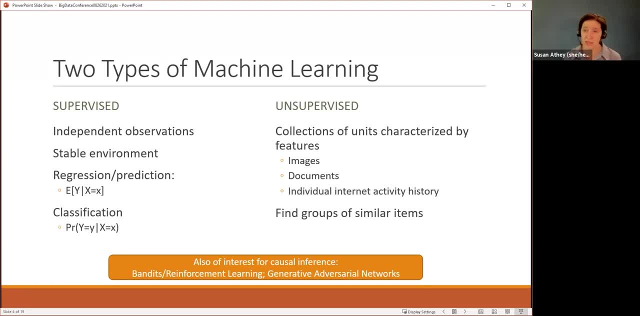 learning in my own teaching. is that actually? the reasons that economists would use unsupervised learning are pretty similar to the reasons other people would use unsupervised learning, So there's no real special like economist version of it, other than the things that I just said. 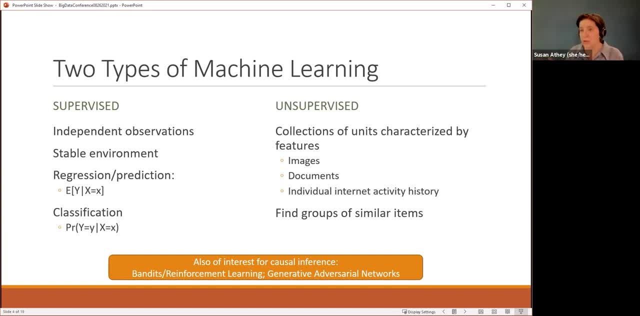 So if you want to do it, you should go read about it, And whichever discipline that is, we'll probably teach you what you want to know, While the approaches that we take to you know classification or regression- are a little bit more often different in the social 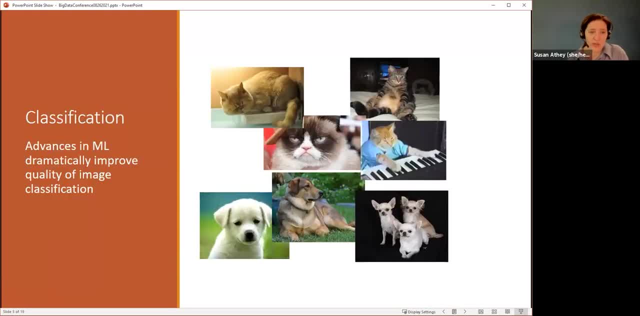 sciences. Okay, So classification? So you know what was the big hot stuff about machine learning and classification Some level. you know the problem of saying, like you know, predicting, a say a zero, one variable like one if it's a cat and two if it's a dog, a zero if it's a dog. 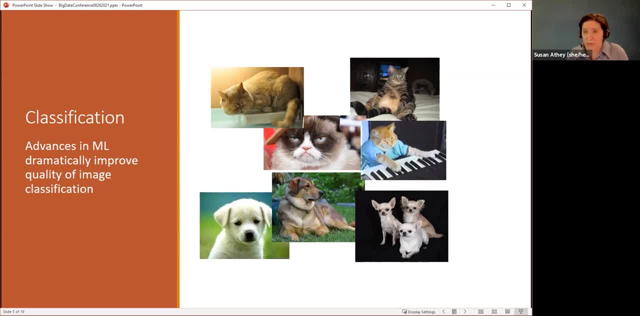 you know that kind of problem we've done Forever Like we. it's called logistic regression and you learned it in your econometrics class. you know, you know how to predict the zero one variable. So what is it? what did machine learning? 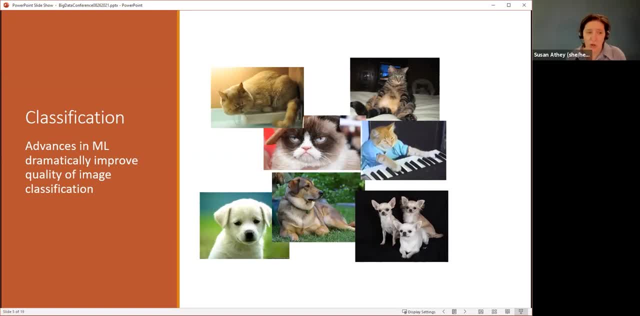 bring to the table in this problem and what was different about it? Well, one of the biggest advances was trying to solve these kinds of prediction problems: predicting a zero, one variable or dichotomous variable, or you know which category something fits in in an environment. 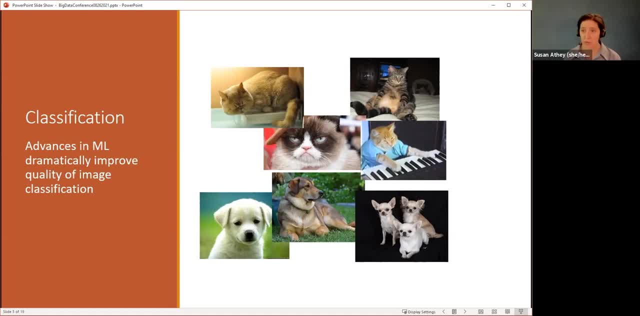 where you had complex right-hand side variables, And so images are this great example And they're one of the big examples where there really has been quite a bit of advance in the last 10 or 15 years. So I've got all. 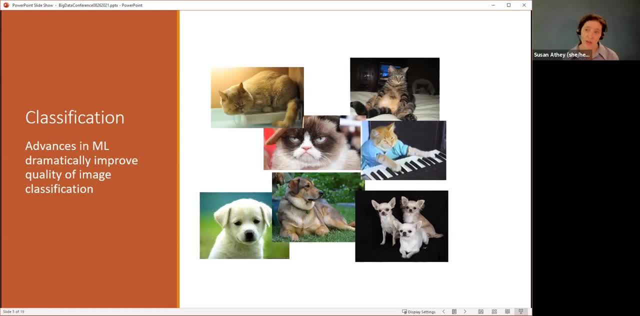 you know, when I first started going to machine learning conferences, I learned that there's lots of pictures of cats and dogs on the screen. So you know, 10 years ago you'd go to a machine learning conference and and I was like what, what is this all about? And that was a time when 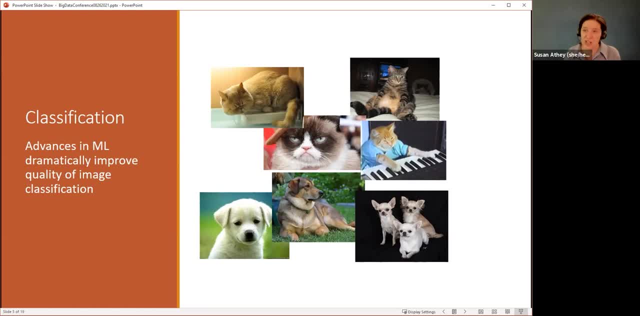 people were getting really excited about the neural nets. So a typical presentation it would be like: oh, I found this better way to train my neural nets And look, I've gotten you know, just a tiny bit better at telling cats and dogs apart. There's actually an interesting 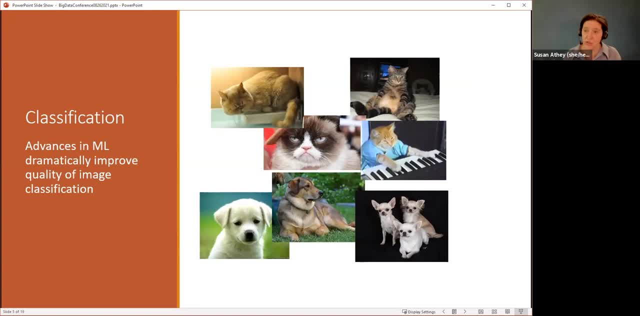 sociological phenomenon that happened here, And one of my colleagues here at Sanford, Fei-Fei Li, helped create this big data set that everybody could apply their methods to. So it was kind of like a horse race. you know, academics are pretty competitive bunch, So you say here's a bunch of 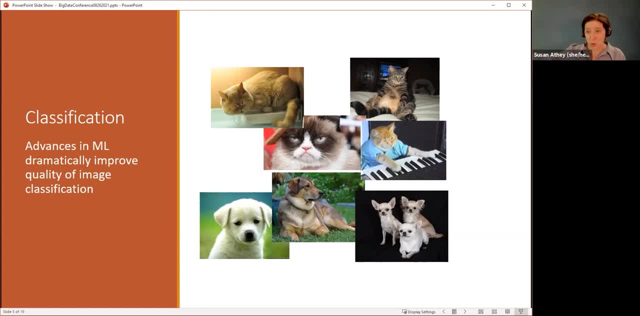 images. It's a really big set of images. And then you're like, oh, I found this better way to train images. And who's the coolest? you know? AI scientist- It's that person who can come up with the very best classification of cats and dogs on this big, big public image data set And they all. 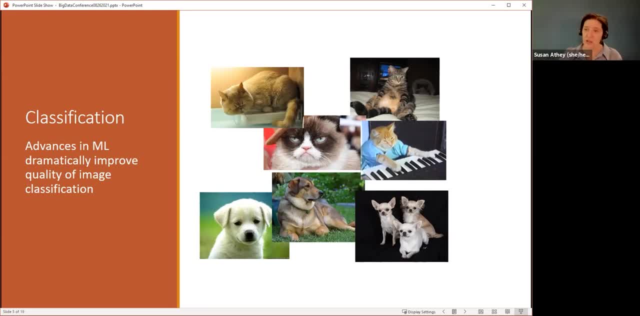 went to town on that. They did a really good job with that And it's kind of an interesting phenomenon where, like having every kind of saying, let's all go to the moon. You know, if you put up a, you put up a common problem and you can all agree on what success is, then you get a very 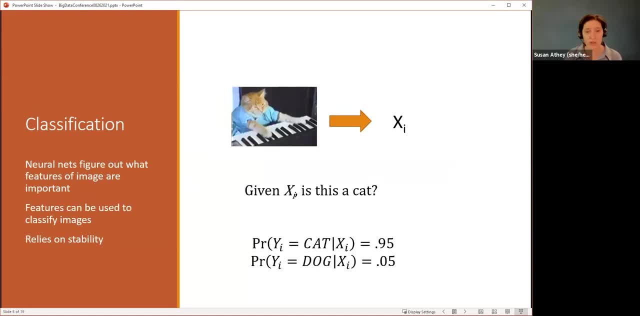 rapid progress towards that goal. So how exactly does this work? Well, how do you go from a picture to a prediction? You can take this image and first of all, just reduce it to to, you know, to zeros and ones, basically. But 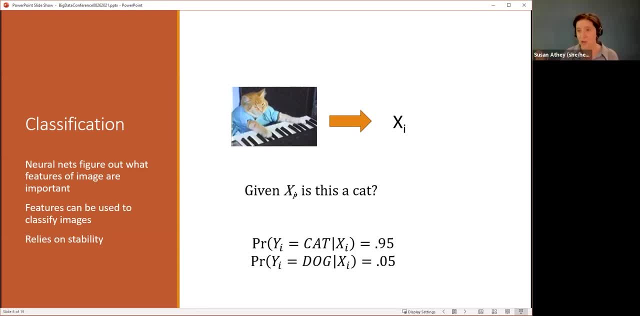 if you think about your. you know you're looking at me on a monitor. that monitor has RGB. You know the way you're seeing my image is that you know each pixel on your little monitor has a certain degree of brightness and different colors. So you can take that image and you can. 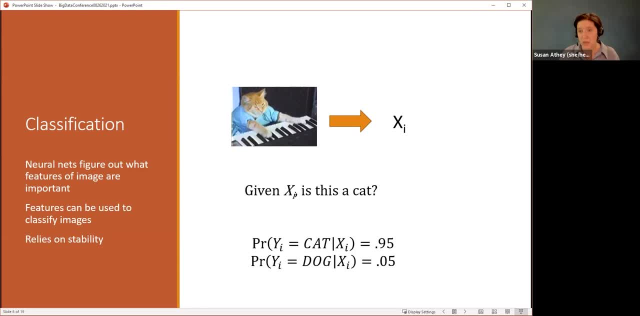 take the image, decompose it into its colors and then describe the image by how bright each pixel is at each point, And so. so that's how you translate, you know, a picture into Xs, which are on the right-hand side of this regression, And then the question would be given those this: 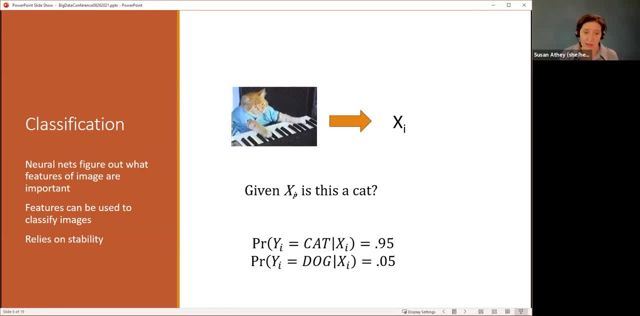 digitization of the image. Now is it a cat, And so when we've traditionally done this in economics, we would. we would build a model that says: you know probability, why I equals cat an X, And once we estimated the model, the output would be a probability. So that's what we've. 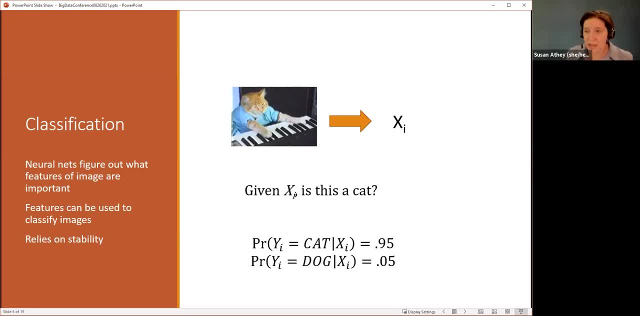 we've typically done in the past. Now, if you were attacking this problem, you know, 15 years ago, as an economist, you never saw anything before you might think. how would I attack this problem? Well, I'd think about the structure of cats. I would think about the shapes of their ears. 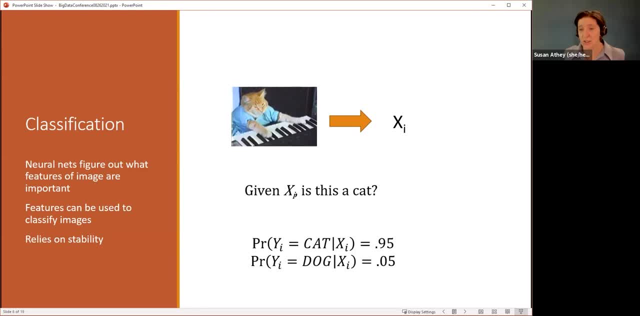 the shapes of their paws, And then I would try to find some way to take those pixels and, you know, first recognize a paw or an ear And then I would try to, you know, classify by pointy ears or round ears whether it's a cat or a. 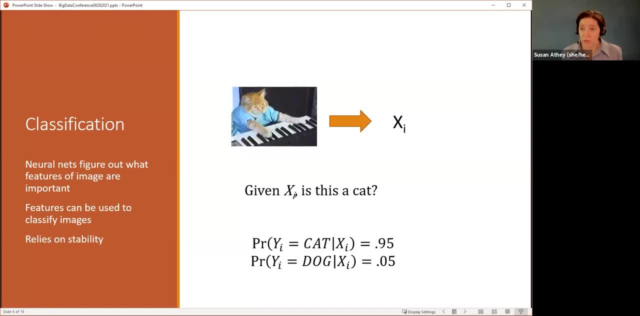 dog. And so you might spend a whole lot of your time first figuring out what those elements were that were different And then, second, trying to figure out how you would recognize them in in an image, right Cause you just have these pixels Like: how do you, how do you even know? 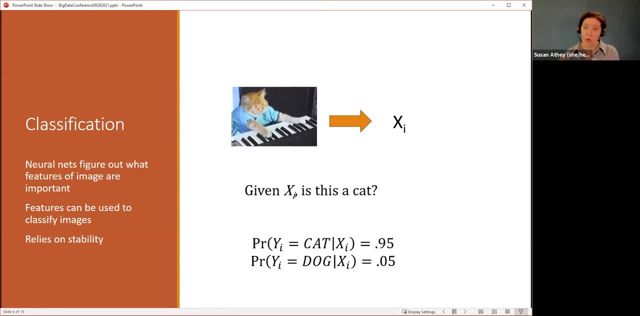 that it's an ear at all, And how do you think about you know, describing the shape of these nearby pixels? So it would be a big feature engineering problem. That's what you call it when you're trying to divide. And the real advance with the neural networks was that the, the algorithm itself figured out. 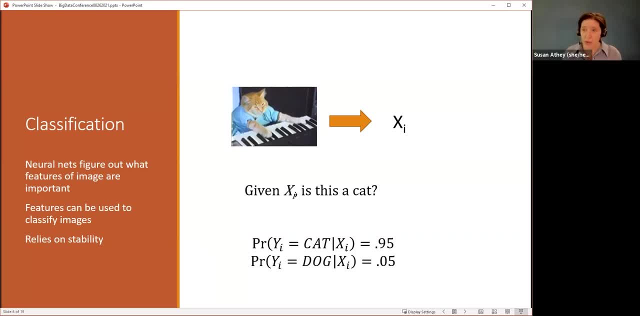 the features. So you would just literally like, just put in the pixels and you wouldn't even have to tell it it was a picture, although it it matters a little bit, you know- but you just put in the Xs and without saying anything else about cats, dogs, ears, nose, whiskers, anything 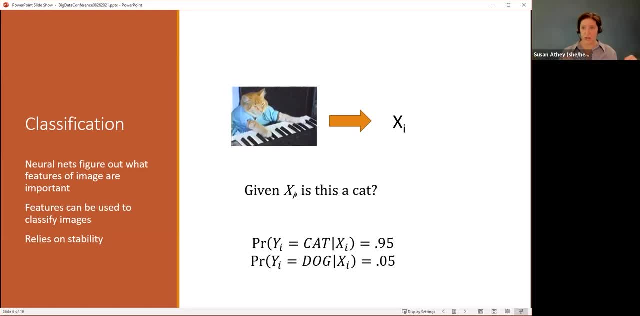 And the neural net just figures out what's important and pops out predictions. So that kind of sounds like magic And I spent a lot of time asking people why it worked and how it worked. And if you check out my videos, I actually have some videos trying to explain. 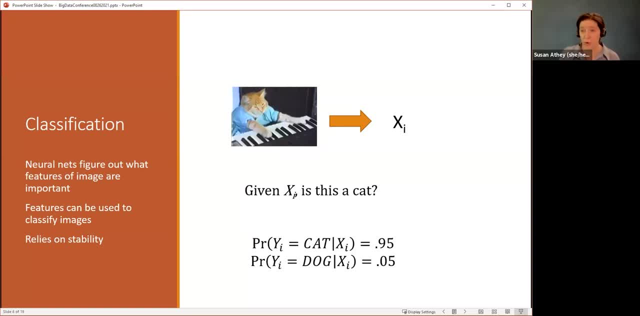 neural nets, my YouTube videos. you know about neural nets and how they work, Although other people's YouTube videos are, frankly, prettier than mine, but you can see mine, cause I'm talking to economists, But I think one of the so what? and? and there's no like like answer, It's just like. 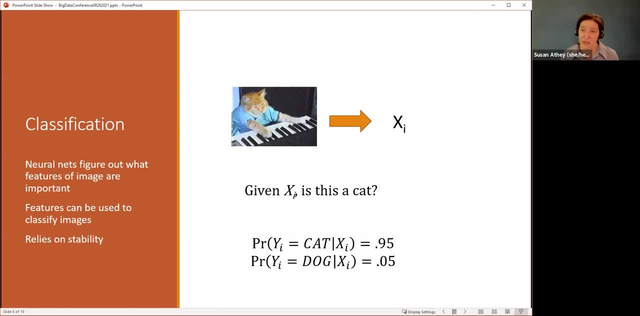 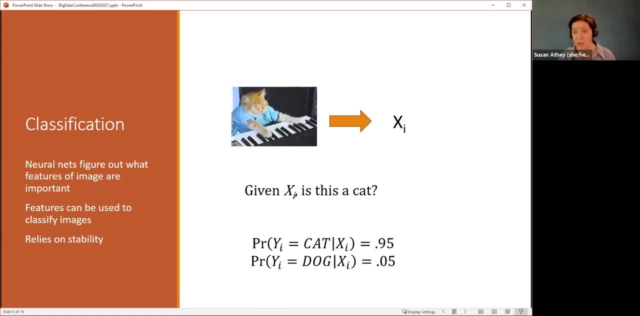 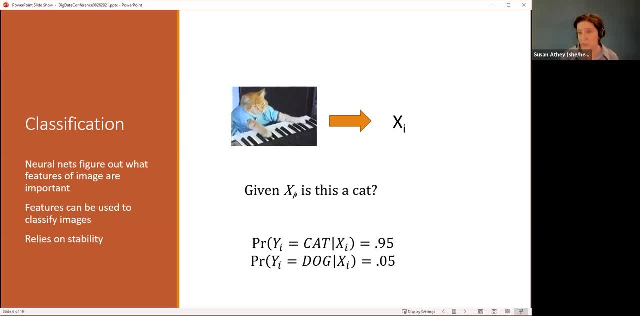 the feature generation to a robot. That's the way I think about it. So the old thing is I would think about ears, eyes and nose and I would try lots of different things, but in the end there's, like you know, if there's however many pixels there are, imagine there's, you know. 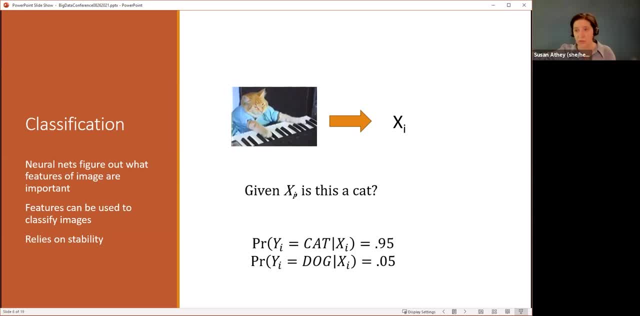 you can represent this picture with a whole bunch of zero one variables or or continuous variables about brightness. There is a limited number of ways you can combine that data into a smaller number of features to build a prediction model. What you do with a neural net? 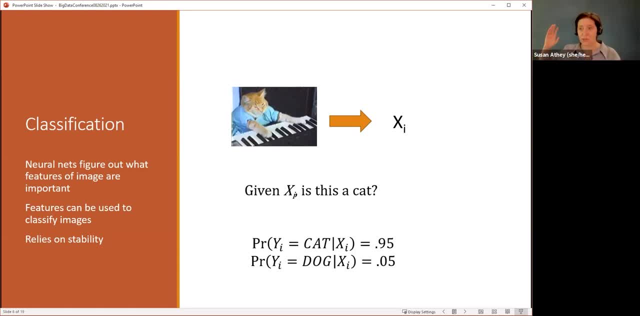 is you just let a robotic research assistant try like a billion different ways to do it, And then it just sees what works and picks the best one. And so then I think thinking about it that way helps you understand what is a really good application for AI or machine learning type of. 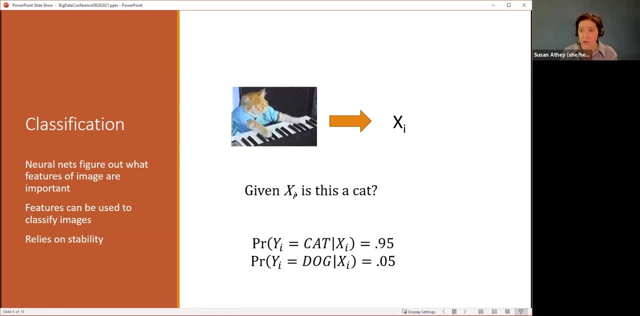 methods. It's a case where there's a clear answer. So I can hold out a test set where there are pictures and there's a label- cat, dog- And then I can let my robotic research assistant try a billion different ways, a billion different functional forms, And then I think: whichever. 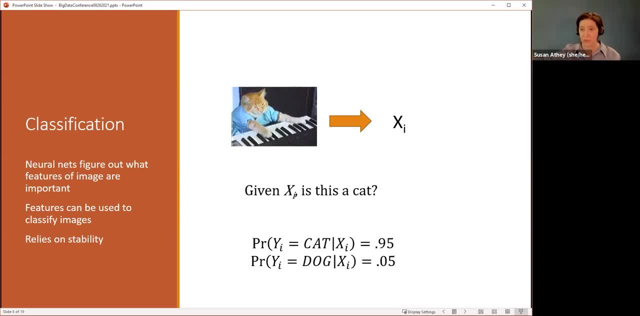 one does the best on my little held out test set, that's the winner. And imagine if you were supervising that research assistant. you wouldn't necessarily care how they got there. but if they have a method that, if you give it another set of pictures, and it does a great job telling cats. 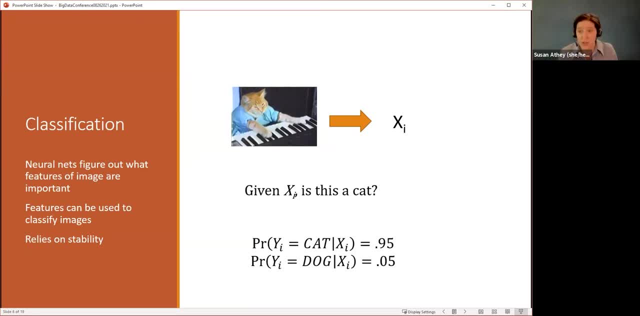 and dogs apart, you're all set. That's all you really need to know. So great applications of machine learning and AI are ones where you can hold out a test set and just assess whether it worked. And so when you think about it that way, then you'd be like, well, where are all the? 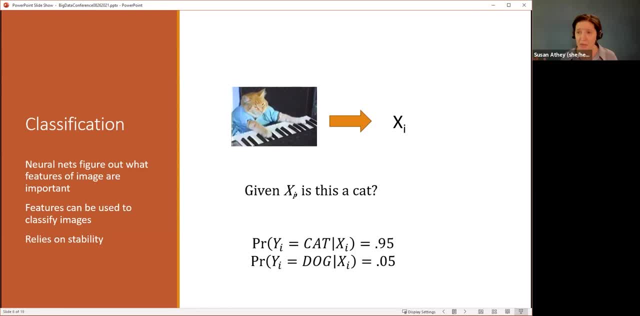 assumptions. Where are these statistical assumptions? They're kind of metrics. They made me do all this math. Why aren't machine learning people worried about all this? Well, you don't need the math if you can just test if something works. I mean it's helpful to. 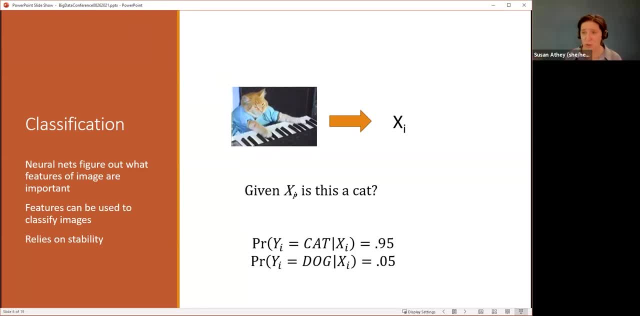 have some intuition about why it works. but frankly, who cares? You can do machine learning without any math. You can just say: you know neural net YX And if it works, it works. That's why you can teach you know 10 year olds to train neural nets. It's not hard. Now there's a lot of. 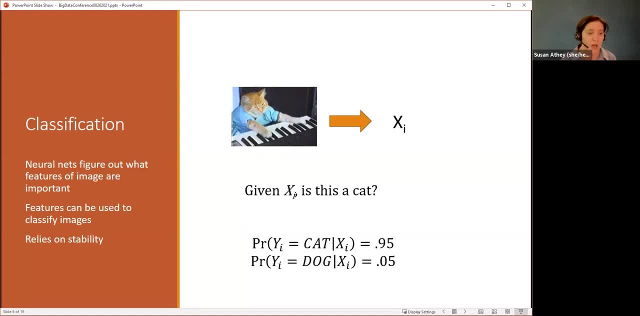 twiddling, but it's not like conceptually hard- Okay, But it does. So that makes it sound like you know there's nothing to it. but when you actually go to use machine learning and practice you often have additional considerations, Like maybe you need the model to not be changed every. 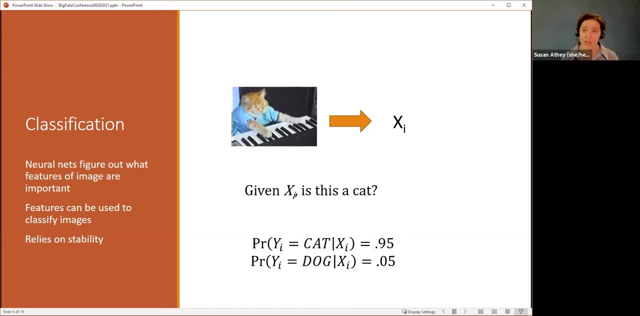 day. Maybe you want a model that's going to work for a long period of time, And so that's where you start to get into the problems of black box models. You know they work great on the problem you have, but you haven't actually. you know you haven't given it any other constraints, So it's. 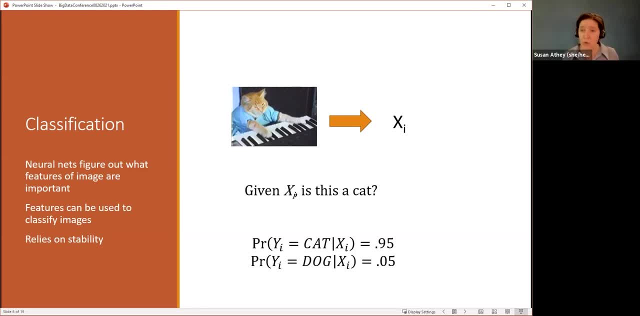 going to pick up everything in the data set you have, even things that might not really hold true tomorrow. So in this particular image I've I've showed you I've got an image of a cat wearing a t-shirt playing a piano. So if this particular week that I gathered my images from had a lot of piano, 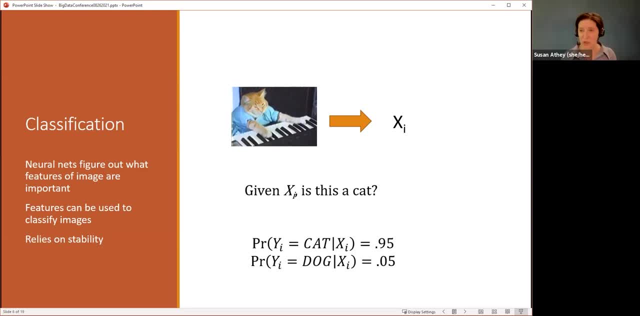 playing cats because like that was the new meme. I guess you know already. you know, back in the day that might've been the thing on YouTube, Now it's the thing on TikTok. If, if suddenly everybody was sharing their piano playing cats on TikTok, then you know the the image corpus. 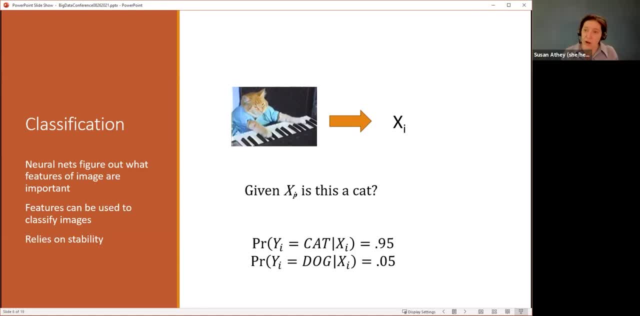 would have, would, would, would have lots of this, And so your, your model, would figure out. the black and white rectangles are good predictions of, of cats, But if the next week, you know, I started a YouTube, a TikTok trend with my piano playing dog, then you know. 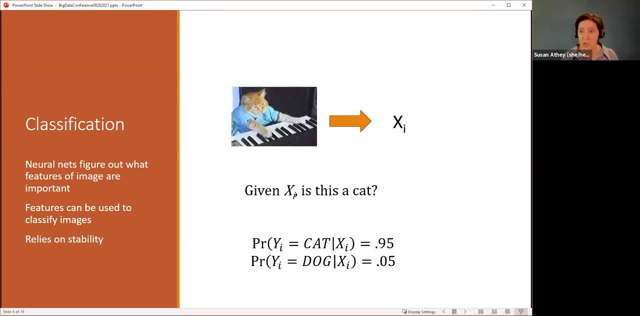 you would, the model might do a bad job. So this is a, this is a limitation. Like the model doesn't prioritize pointy ears over t-shirts and pianos, It- just like whatever is correlated with being a cat is is going to be predictive of a cat And in fact you know it's going to pay attention. 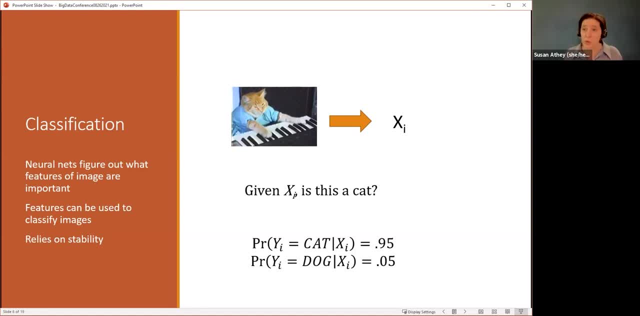 To that stuff, because the the model that ignores pianos would get beaten by a model that included pianos in a dataset where there were more piano playing cats. So, like you're going to use everything, That's what's going to happen. You know you're going to use everything that's. 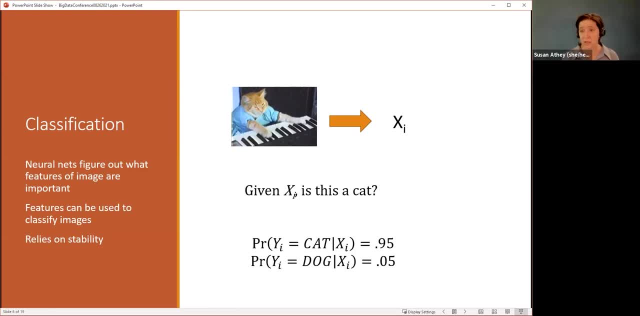 predictive. So that's a strength and a weakness. It works well at a moment in time, it exploits everything possible, but it doesn't have any kind of common sense about what might be important or generalizable or stable. So here's another example. This is from a McKinsey marketing brochure. 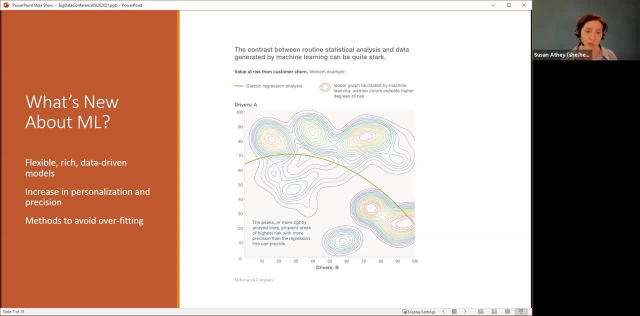 where the idea was to try to use data to classify whether customers are going to churn or not, whether they're going to quit, And so here this shows the old version is like a classic logistic regression is the green curve, And so it's basically saying that drivers A and drivers 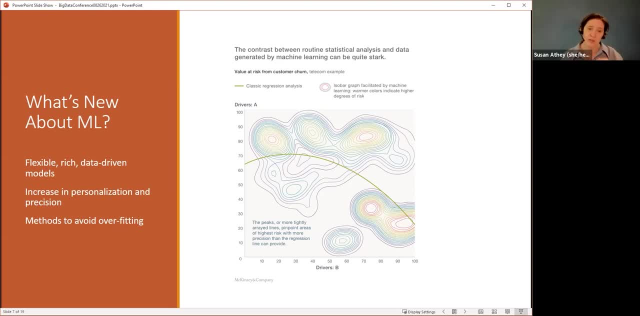 B are the X variables And in the simple model things in above the curve would be predicted to churn and things below the curve would be predicted not to churn. Then they're showing. this kind of topographical map is the example of what you would get from a fancy machine learning. 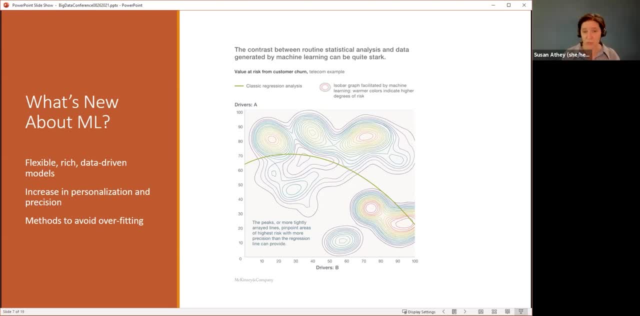 method. So this might be a really good predictor, but if you actually tried to generalize or use this to gain insight, you would realize it doesn't necessarily work as well, Because if you hold drivers A constant, say at 80, and increased drivers B, it's saying the probability of churn. 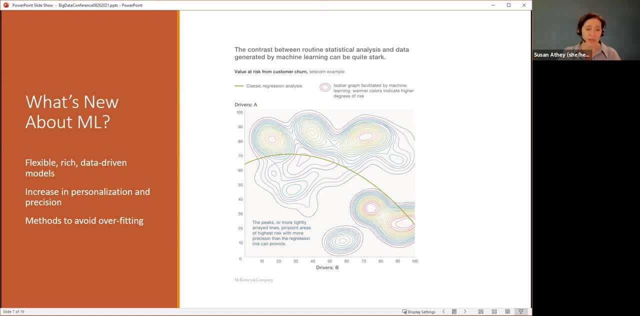 goes up and down, and up and down, and up and down, Like I don't know what the heck drivers B is, but there's probably isn't any variable like that where that's truly the partial relationship with respect to B. So why do you get this funky, complicated picture? 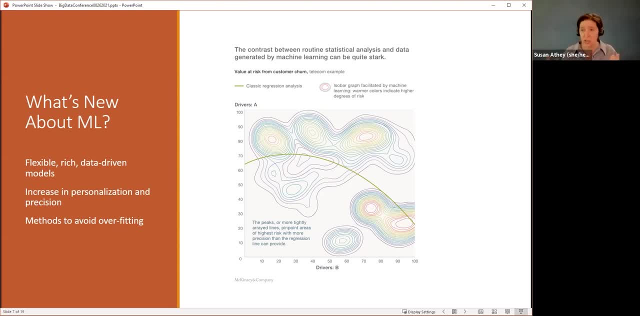 Well, it's because there's lots of covariates and they all have this very complicated joint correlation structure, And so you know, in the background, as drivers B changes, a whole bunch of other stuff is changing and you have this complicated nonlinear model that's exploiting. 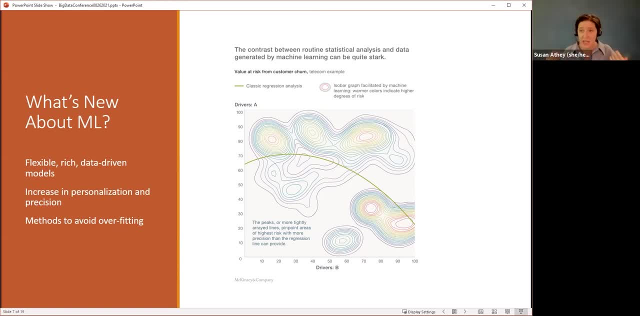 very fine details of the joint distribution of all the Xs And that works well in the dataset we have. but if anything changes about the joint distribution of the Xs then the whole thing could break. So this is a potential weakness of these models And I actually have a line of research in machine. 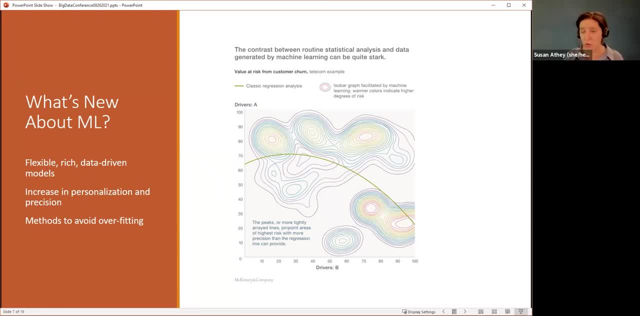 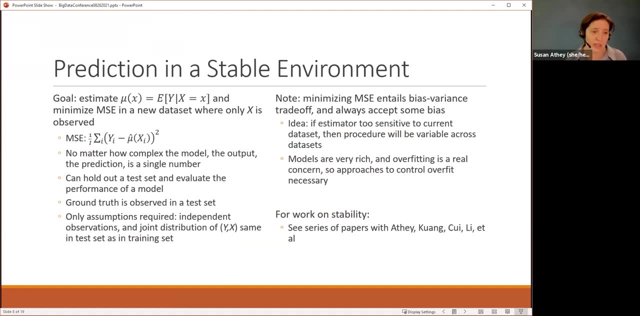 learning that published in AI journals about trying to reduce the dependence on these high dimensional joint correlations. So then just to kind of pull this together: prediction in a stable environment is the problem that's solved by supervised machine learning. The goal is just to build a model that comes up with a good prediction, and you want to minimize means. 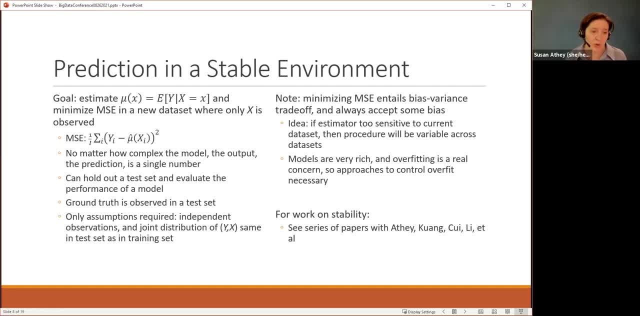 squared error in a test set And you can just tell whether it works by checking what happens in a test set. A few observations is that minimizing means squared error actually entails a bias variance trade-off and you're actually always going to want to accept some bias. 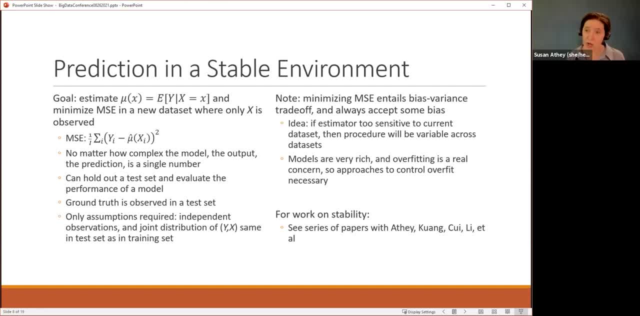 So you're not. in econometrics class. they often taught you that you like OLS is blue unbiased. That was one of those. that was the U in blue. if you forgot it already, And you know, you had to spend a lot of time memorizing the proof. 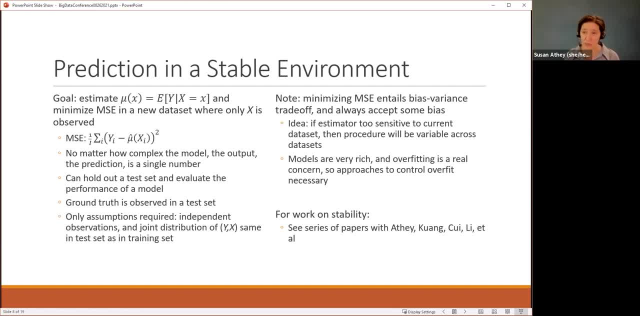 that, like OLS, was the best linear unbiased estimator, But they didn't tell you in class, unless you took a very modern class. they didn't tell you that actually having an unbiased estimator comes at a cost and actually it potentially would give you a worse predictor. 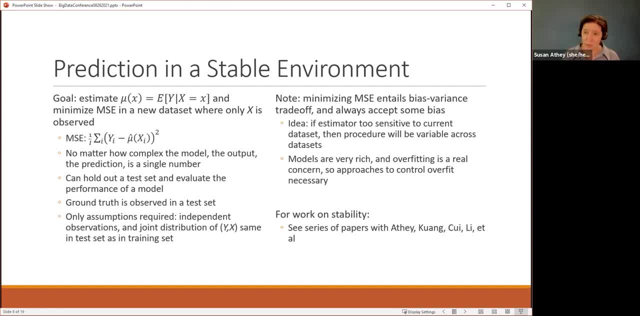 in a test set. Now it turns out that being unbiased is kind of free if you have a small number of parameters you're estimating and a very large data set. But the difference with machine learning is that when you're doing a test set, you're going to have to go back and 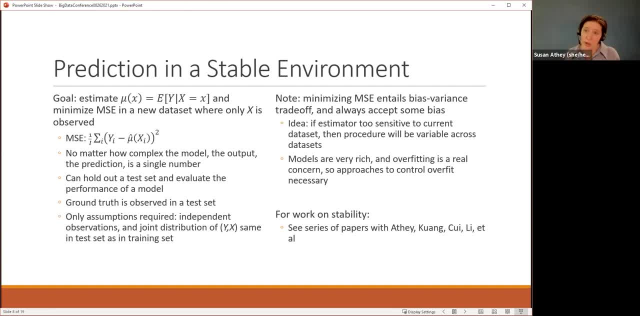 look at a lot of different models, And so we actually try lots of very rich models, And so we push the limits, We make the models richer and richer and richer. And so in that world, being unbiased does come at a cost, because if you have a really rich model, you're always going. 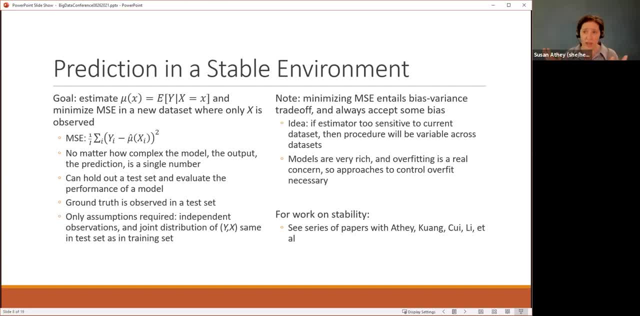 to overfit. Like if I tried to predict everybody in the class, like whether they had coffee or not, if I- literally there were 40 people in the class and I used a 40-dimensional model, I could predict perfectly whether you had coffee or not in the break, right. But if I went to the next class, 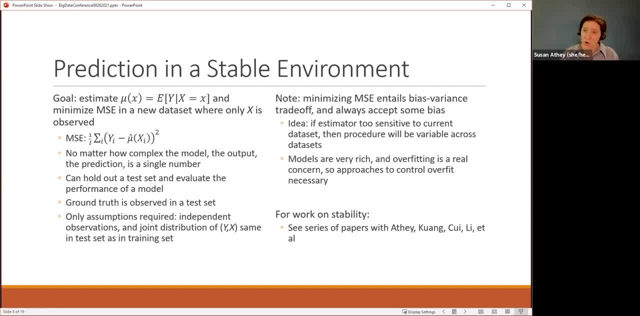 tomorrow, I could predict perfectly whether you had coffee or not in the break. But if I went to the next class tomorrow, I could predict perfectly whether you had coffee or not in the break. right, So my model would be terrible. So when you have very rich models, there's a trade-off between 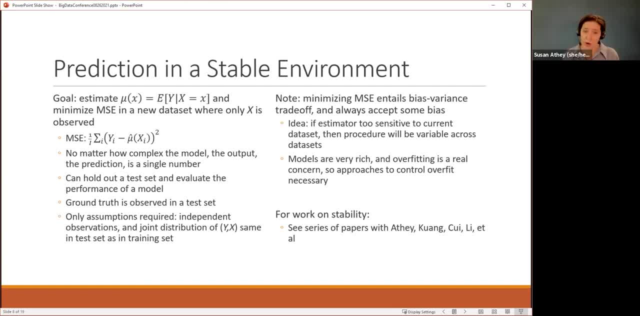 predicting well in the data you have and generalizing elsewhere, And the optimal model is somewhere in between. So the models are very rich. Overfitting is a real concern And a big part of the machinery of machine learning is figuring out the right thing, right way to. 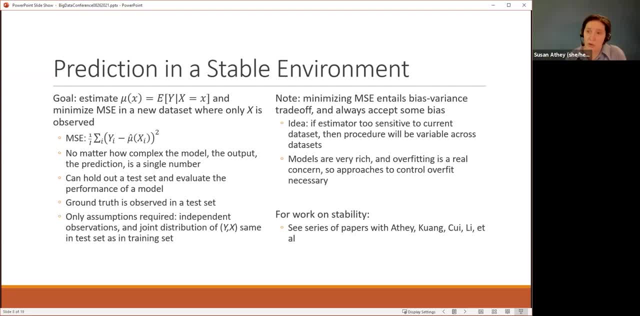 optimize that And the most generic machine learning models are optimized for MSE. But one of the things that I've done in my work is modify the objective And I've done a lot of machine learning models to try to make them more optimized for other objectives, things like 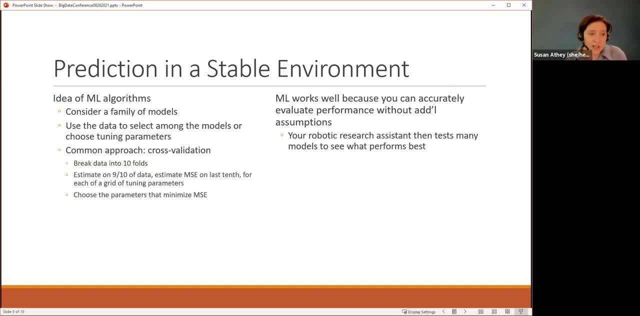 causal inference. So the idea of machine learning algorithms is: you consider a family of models. you use the data to select among the models, which is called choosing the tuning parameters. So the family includes simple models or rich models Like an OLS. it might be three variables. 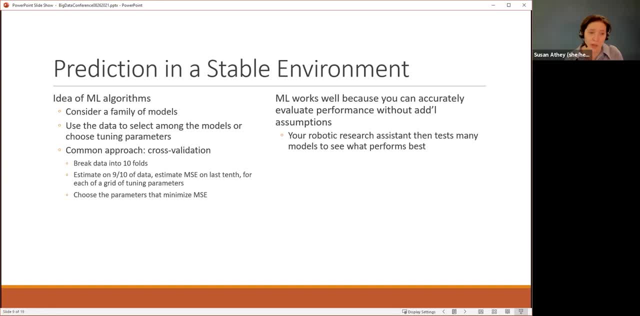 or 100 variables. It would be all in the family of OLS regressions. You use cross-validation to choose which might be. for example, you might break the model. you might break the model. you might break the data into tenfolds. You estimate a model on nine-tenths of the data. 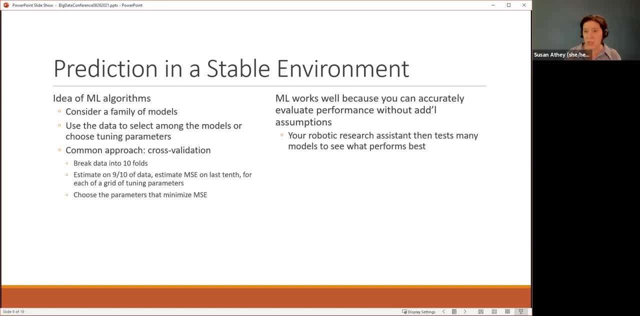 Look at the mean squared error on the last tenth And then you see how rich a model actually gets the best mean squared error. And machine learning works well because you can accurately evaluate the performance without additional assumptions. Your robotic research assistant tests many models to. 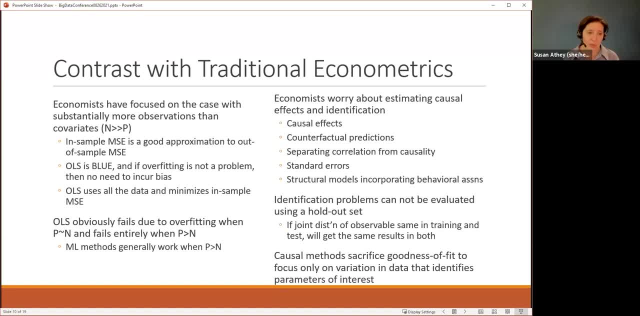 see what performs the best. To contrast that with traditional econometrics: in traditional econometrics, economists focus on the case-by-case ratio, So you have a model that's going to be a good approximation to the out-of-sample mean squared error. In contrast, economists typically 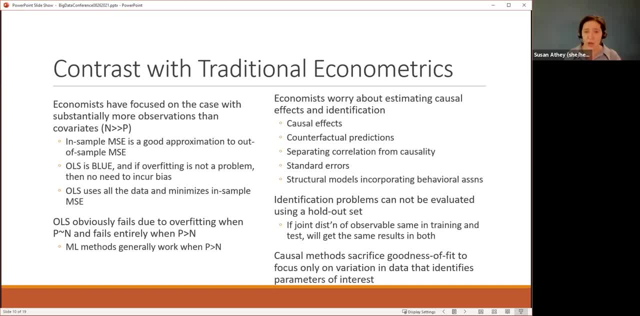 imagine, at least, that they have a fairly simple model and they worry about things like estimating causal effects or identification. So we want to know what was the effect of having more immigrants come into Miami? What was the effect of changing the minimum wage? What were the effects of COVID-19?? 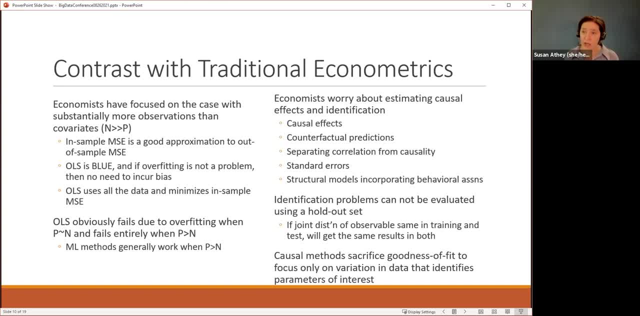 What were the effects of COVID lockdowns? These are all different kinds of policy questions you might answer. And then we're often interested in counterfactual predictions like what would happen if we had another lockdown? What would happen if we had gotten vaccinations earlier? 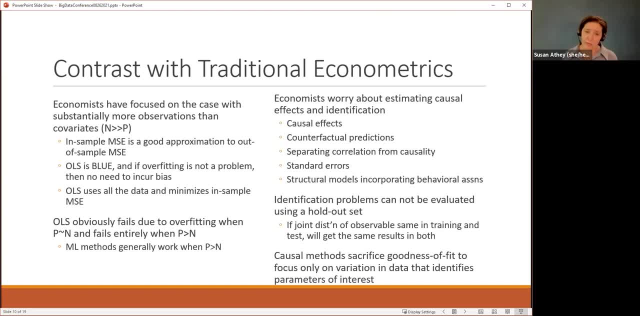 Things like that. And then the empirical problems we worry a lot more about are separating correlation from causality. We also worry a lot about standard errors. Even if we run an experiment, we're worried that our result might just be due to sampling. 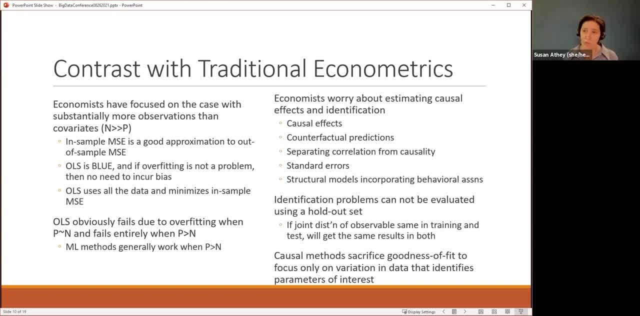 It might not generalize very well. We also try to incorporate behavioral assumptions Or, if we're looking at some more complicated macro model, we may not have enough data to really pin everything down, So we're going to have some combination of behavioral assumptions and calibrated parameters. 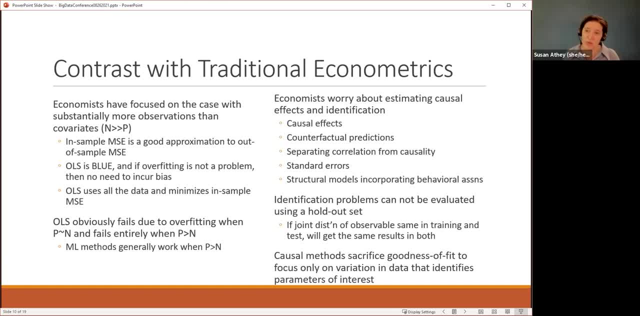 and functional forms that help guide us to have a data-driven theoretical model. So a few observations on that, just to kind of close the loop here. Identification problems which cannot be evaluated using a holdout set. So identification is the question. if I had infinite data, would I even be able to? 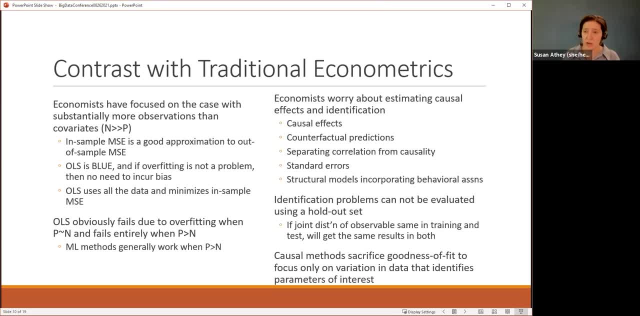 answer my question, And we put a lot of emphasis on that in economics, especially in micro. That's not something that you can figure out in a test set. So a simple example would be like: suppose that you were looking at the impact of price on sales. Well, if people typically 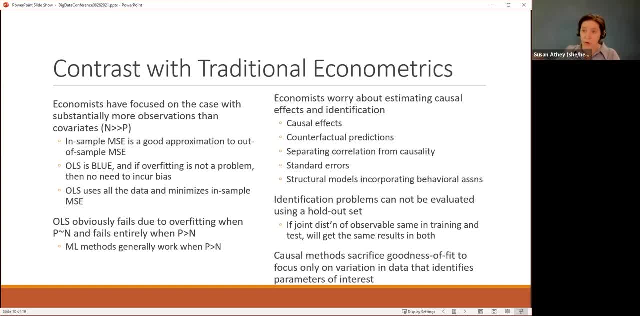 raise their price in peak times, then prices and quantities would be positively correlated, Because when there's a big demand shock, the firms raise their prices. So you would see lots of sales at a time with high prices. That positive correlation between prices and quantities. 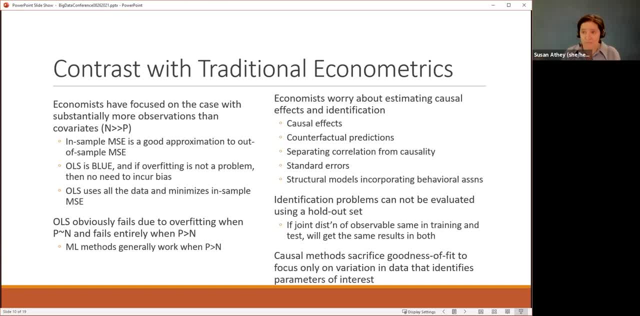 will be true in a training set. It's true in a test set. Splitting your data or having held out data doesn't fix that problem at all. Instead, we learn that you need something like a natural experiment or some kind of experiment. And if you're looking at the impact of price on sales, 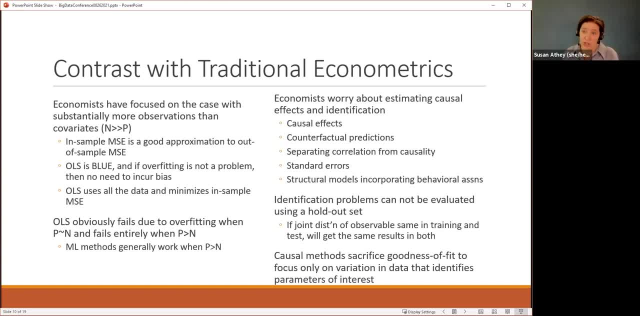 you're looking at the impact of price on sales, So you need to have some kind of exogenous variation or some kind of supply shock to be able to understand the relationship between prices and quantities. That type of logic was not there in traditional machine learning at all. 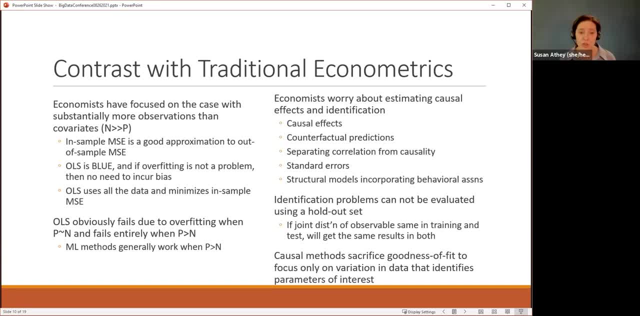 Wasn't really part of the textbooks or the framework, So the traditional supervised machine learning kind of classes you would take. So causal methods typically sacrifice goodness of fit in order to focus only on variation in the data. that identifies parameters of interest, And it's just a very different way to think about it. 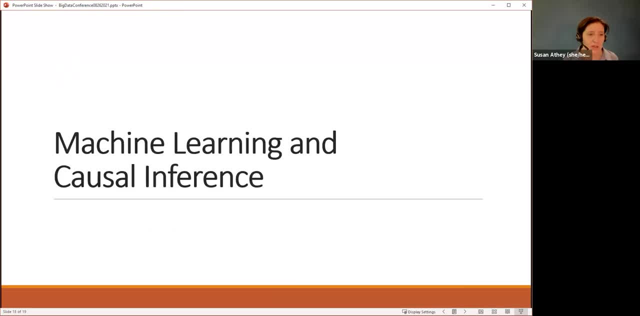 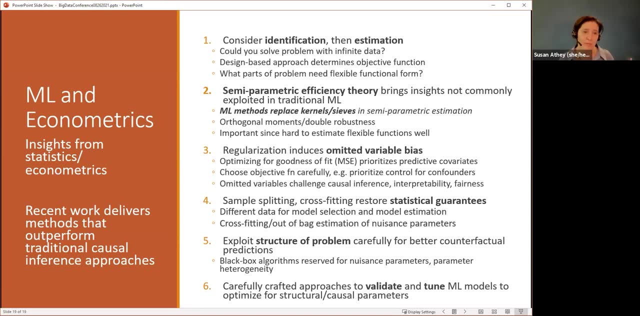 I actually skip ahead to kind of a little bit of a kind of summary of how we've brought together machine learning and econometrics in the causal inference literature. These are like kind of six sort of takeaways. We first have said that machine learning is actually more about solving estimation. 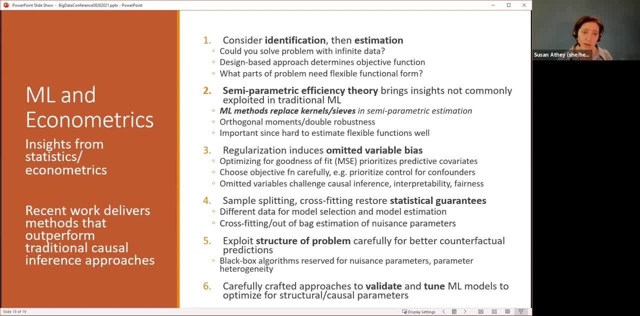 problems and good functional forms. So, as an economist using them, you might first consider identification. What would you do with infinite data? And then machine learning? you might first consider identification. What would you do with infinite data, And then machine learning. 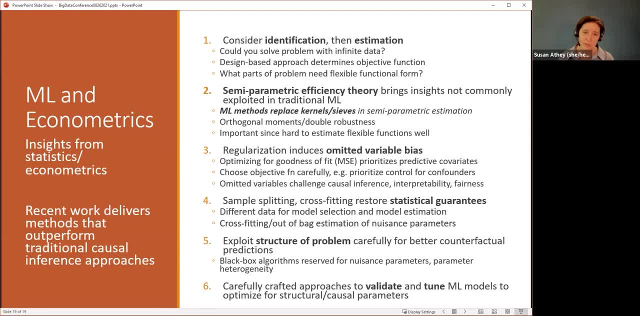 you might first consider identification- What would you do with infinite data? And then machine learning is going to be more about figuring out what the best functional form is. A second point, and this is more for the econometricians: is that actually we have? 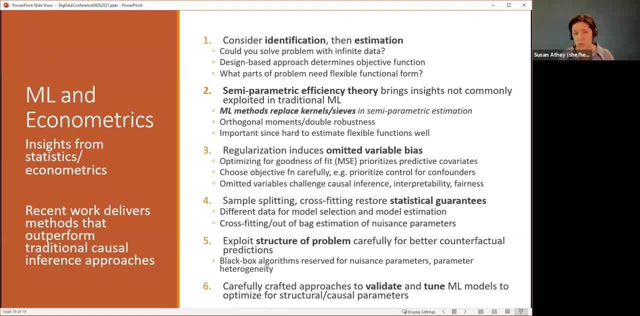 a huge literature already that says what you should do with semi-parametric models or, when you want to be flexible functional forms. We had great theory. We just had bad practice, Like the models didn't work, So the machine learning can come in and have sort of better. 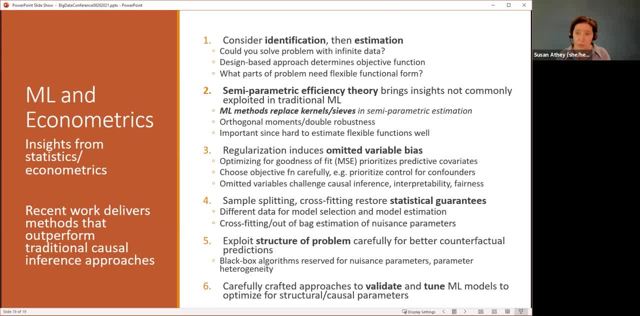 performing computational methods and functional forms and so on. But actually the theory is helpful And we actually collectively have pushed forward machine learning theory by bringing in ideas from semi-parametric efficiency theory. Once we change the question away from just prediction and make it towards 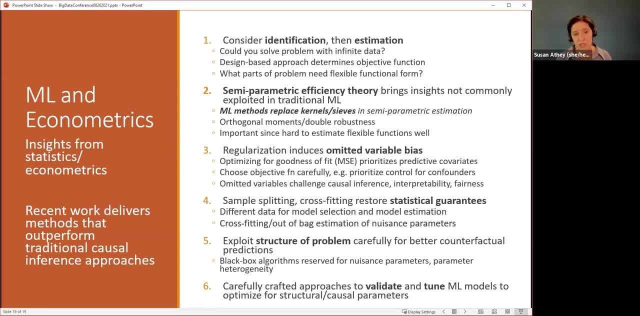 estimation. A couple of other points. regularization can introduce omitted variable bias. That means when we do this model selection, sometimes we can throw away variables that might be important to control for if we have a more causal approach. So that's another reason we just 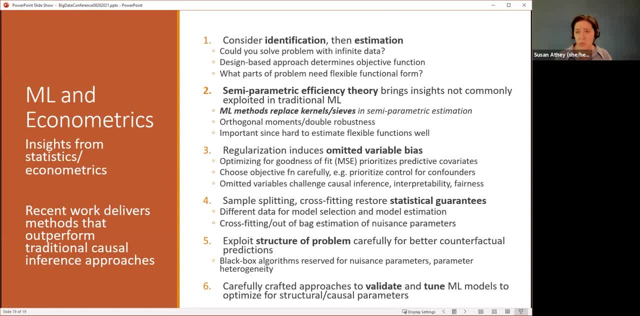 don't throw the kitchen sink at a causal model. Instead, what we do is we break the problem apart. Thanks for having me, Elizabeth. Thank you, I think there's a couple questions here that I want toа apart. give some parts of the problem to machine learning, but change the objectives in the way. 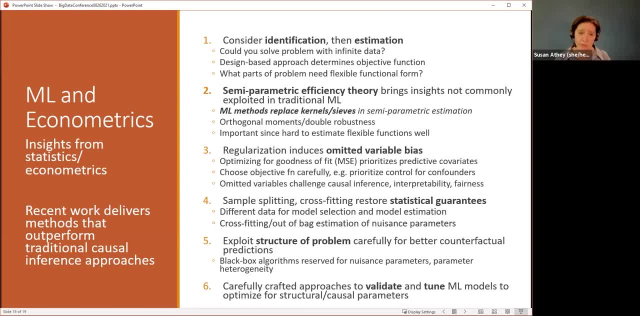 that we optimize the problem to solve causal problems. Machine learning hadn't done much about sample splitting or crossfitting. There were some techniques that we've introduced coming from the statistical theory perspective, And we've also tried to show how you can exploit a structure of 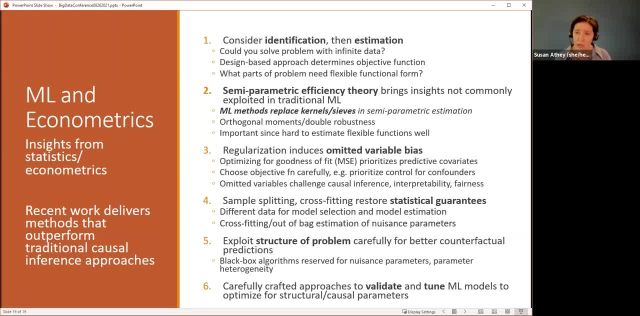 a problem carefully to have better counterfactual predictions. So bringing in some ideas from either structural economics or, or you know, aspects of a problem that are where you were. in economics, we had already put a lot of effort into finding the very best way to estimate a parameter. 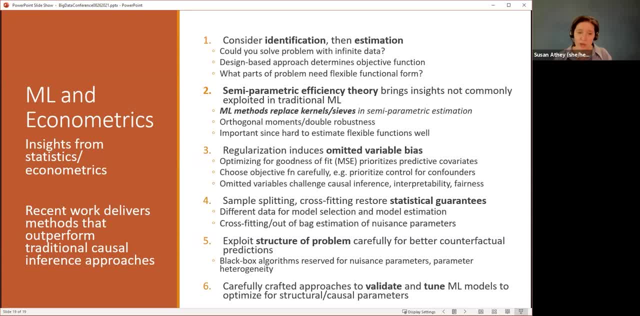 Now we just throw machine learning into kind of the non parametric parts of that problem. And finally, it's actually pretty hard to test whether your approach works with causal inference, because people don't have causal effects stamped on their forehead. So I don't know. 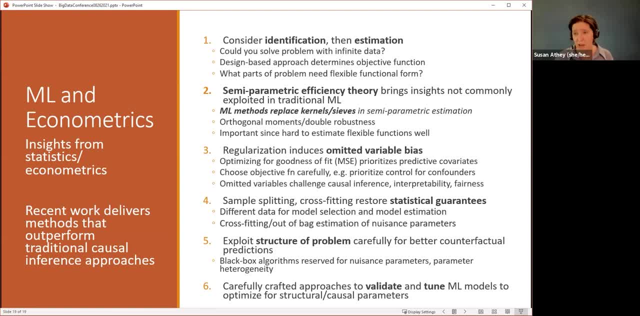 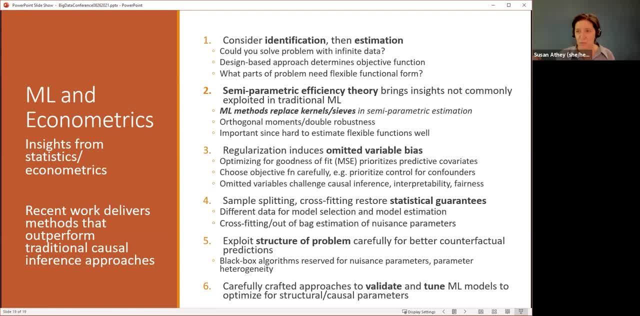 in the break or not, He had a cup of coffee. so he's bright eyed and bushy tailed. But what if he hadn't? So I can't just look at his outcome and know the causal effect of coffee. So we've had to.